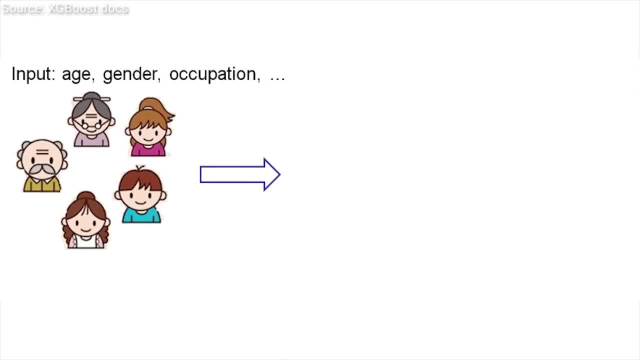 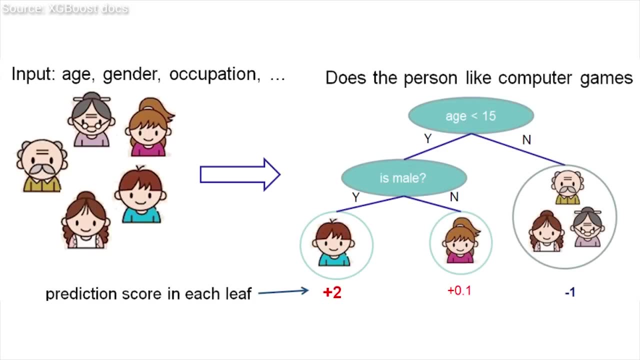 to find out whether they like computer games or not. Note that this is a toy example for educational purposes. We can build the following tree: If the person's age in question is over 15, the person is less likely to like computer games. 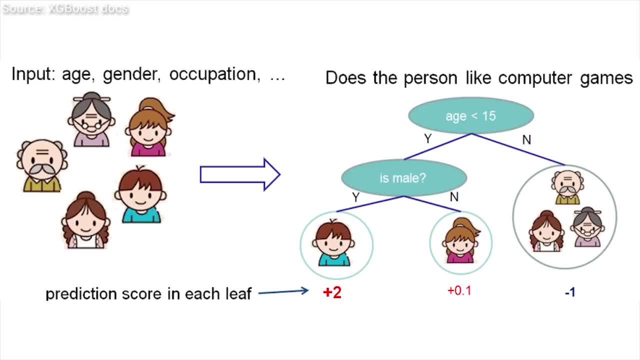 If the subject is under 15 and is a male, he is quite likely to like video games. If she's female, then less likely. Note that the output of the tree can be a decision like yes or no, but in our case, 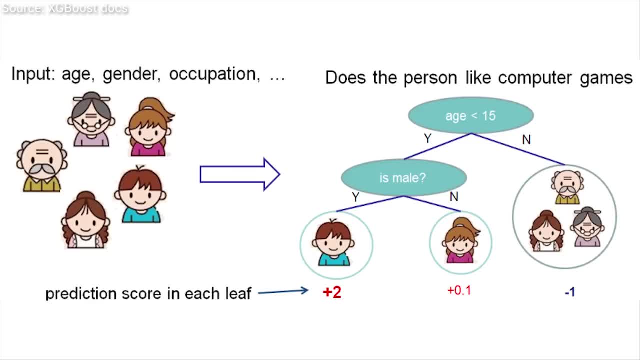 we will assign positive and negative scores instead. You'll see in a minute why that's beneficial. But this tree was just one possible way of approaching the problem, and admittedly not a spectacular one. A different decision tree could be simply asking whether this person uses a computer. 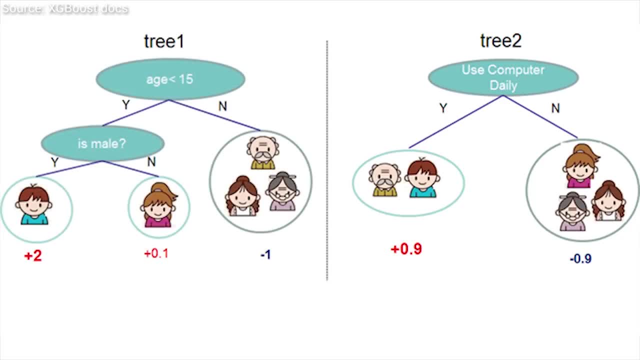 data. Individually these trees are quite shallow and we call them weak learners. This term means that individually they are quite inaccurate, but slightly better than random guessing. And now comes the cool part. The concept of tree boosting means that we take many weak learners and combine them into 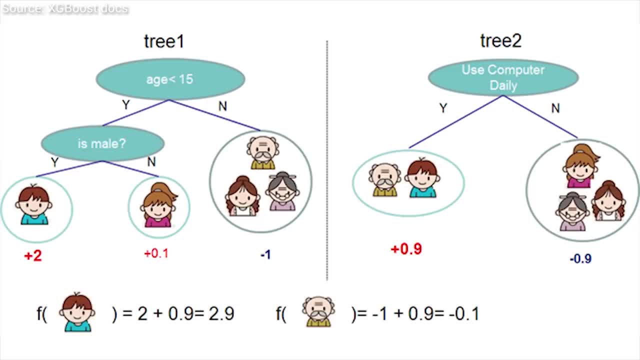 a strong learner. Using the mentioned scoring system instead of decisions also makes this process easy and straightforward to implement. Boosting is similar to what we do with illnesses. If a doctor says that I have a rare condition, I will make sure and ask at least a few more. 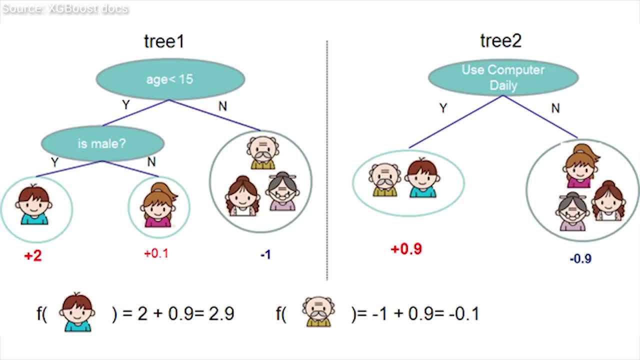 doctors to make a more educated decision about my health. The cool thing is that the individual trees don't have to be great If they give you decisions that are just a bit better than random guessing. using a lot of them will produce strong learning results. 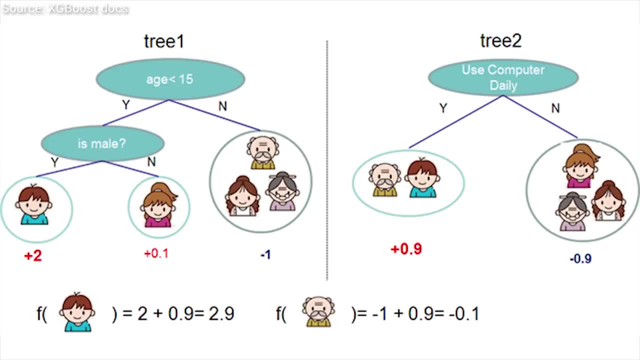 If we go back to the analogy with doctors, then if the individual doctors know just enough not to kill the patient, then we can make a better decision. A well-chosen committee will be able to put together an accurate diagnosis for the patient. An even cooler, adaptive version of this technique brings in new doctors to the committee. according, 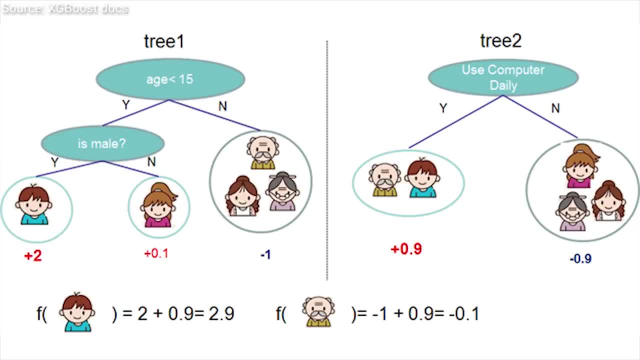 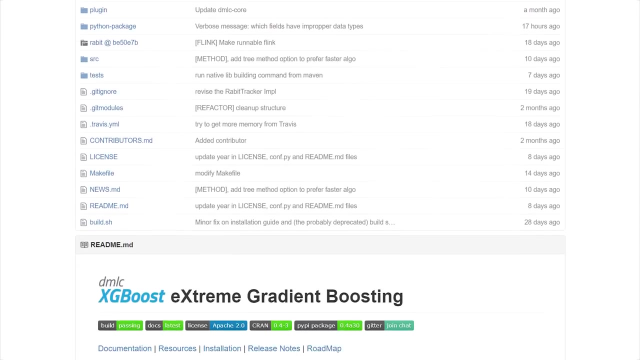 to the deficiencies of the existing members. One other huge advantage of boosted trees over neural networks is that we actually see why and how the computer arrives to a decision. This is a remarkably simple method that leads to results of very respectable accuracy. A well-known software, for example, has been using boosted trees for many years.